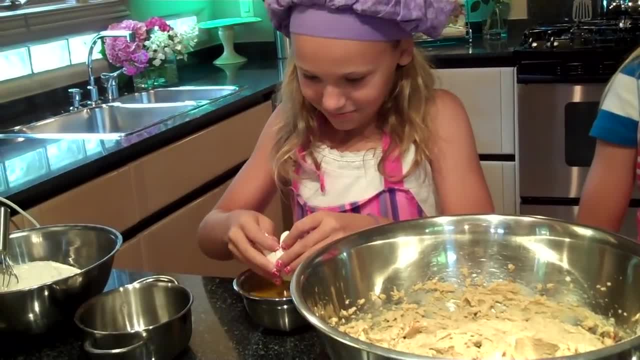 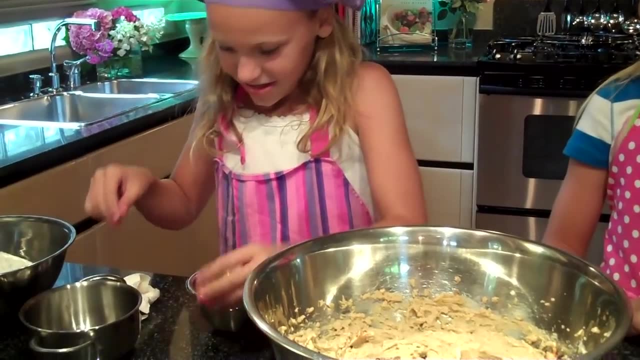 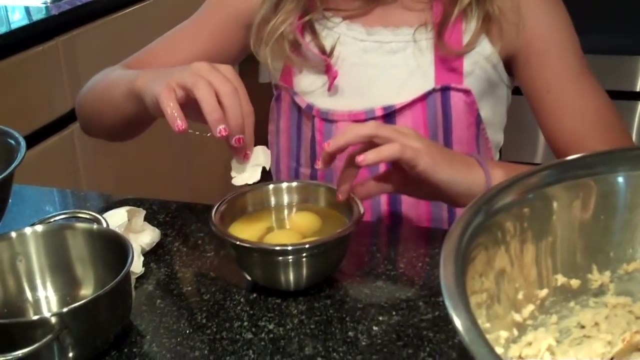 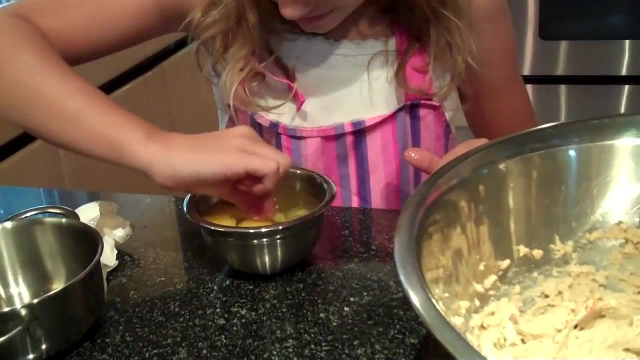 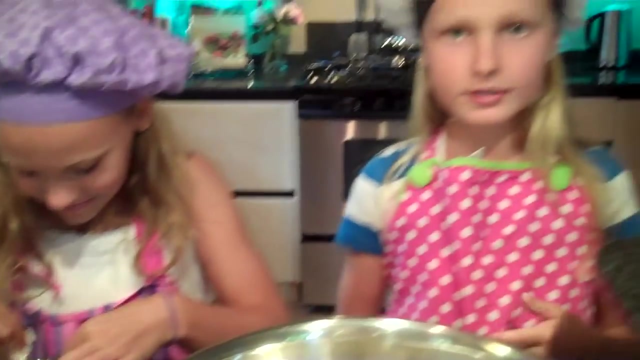 Oh, there's a shell at the bottom. A good tip for getting shells out of the eggs is taking a different part and scooping it out of the bottom. If you've never heard eggs, eggshells attract to the other eggshells, so it'll pick that. 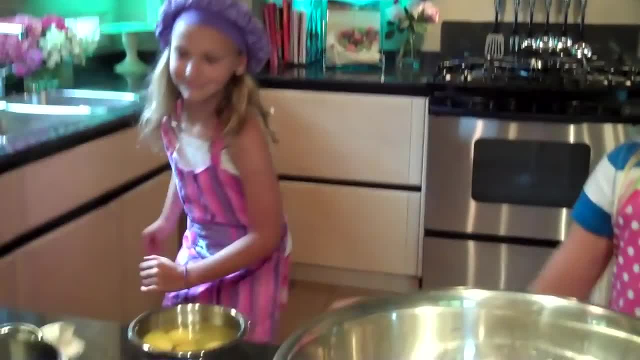 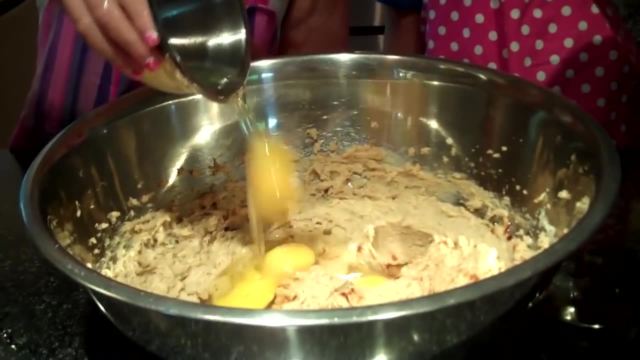 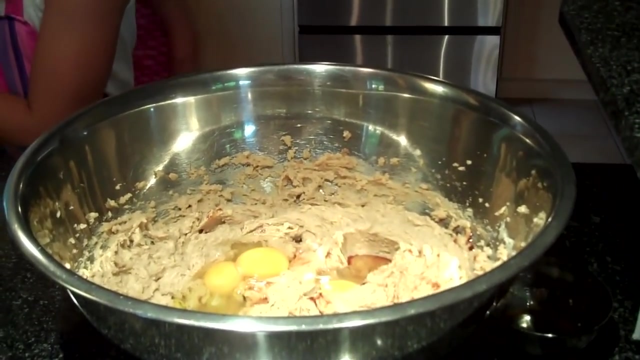 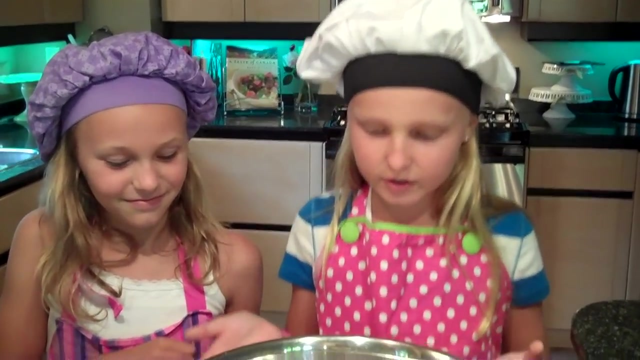 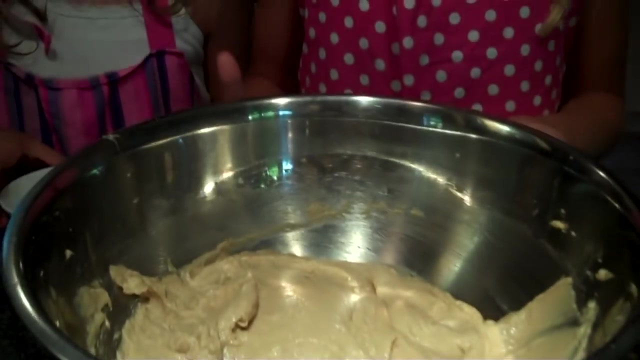 up and you're ready to go. So Molly will now add this to that: Four eggs. Now we're going to beat it. So I'm going to grab the beater and start beating. This is what your dough should look like After you've mixed in the eggs and the vanilla. So, as you can see, Now Molly will add baking. 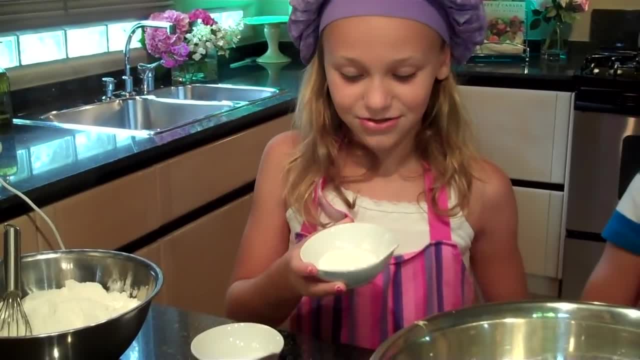 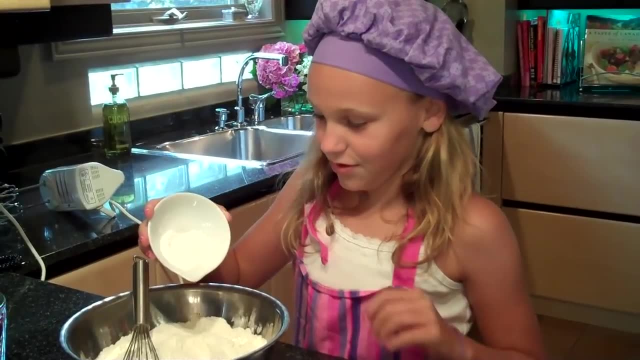 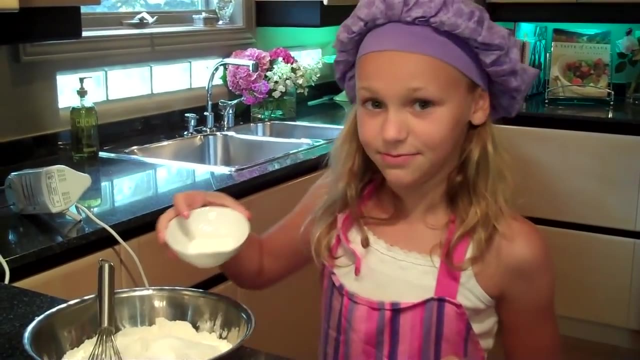 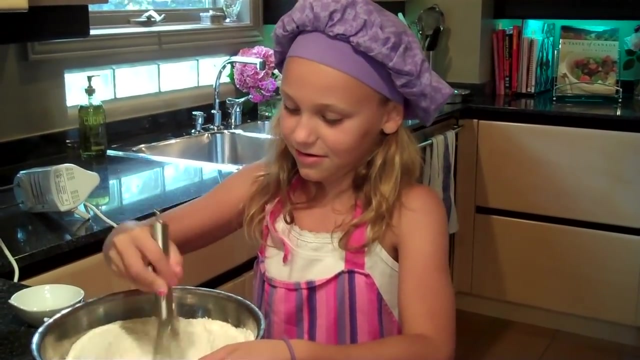 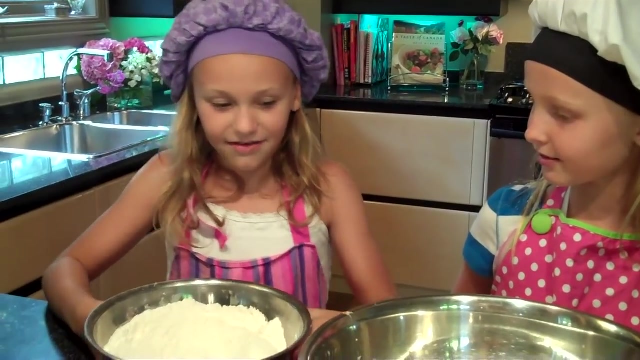 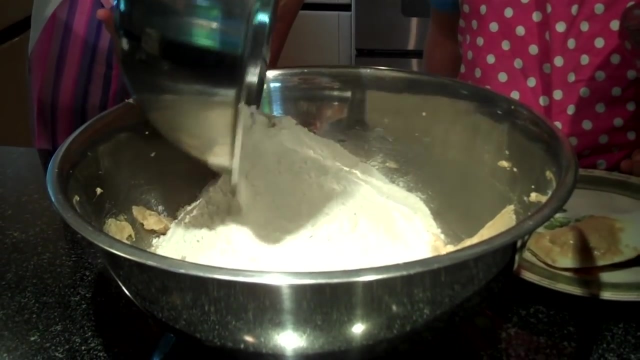 soda and salt to some flour. You add two teaspoons of baking soda into your four and a quarter cups of flour, and then, after that, two teaspoons of salt. Now I'm going to whisk that together. Now I'm going to add my flour into the wet ingredients. 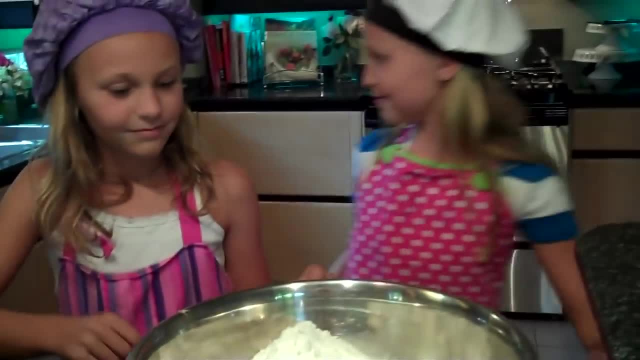 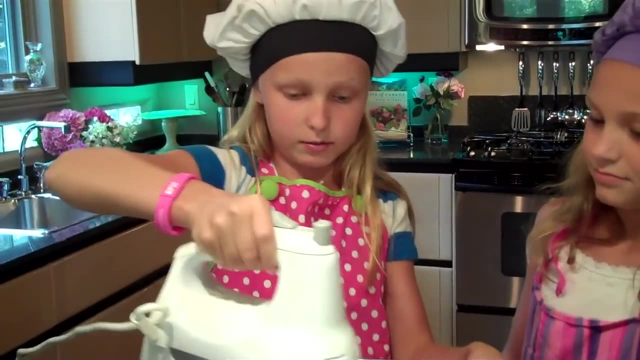 Now we're going to start beating our dough, So let's get the beater. And a trick is is you mix it in so the flour doesn't stick to the bottom of the bowl. So you're going to beat it, You're going to mix it in so the flour doesn't go all over the place. See, 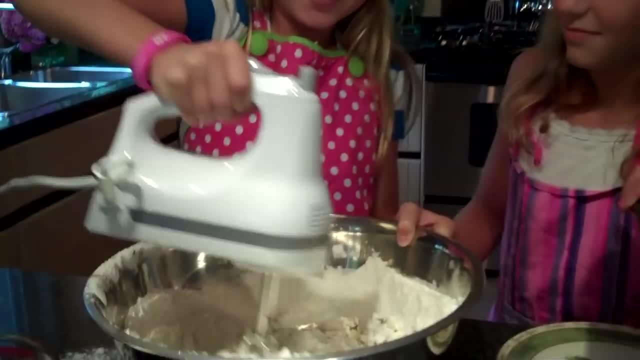 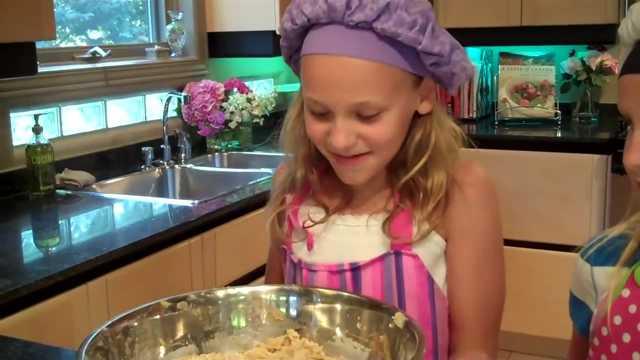 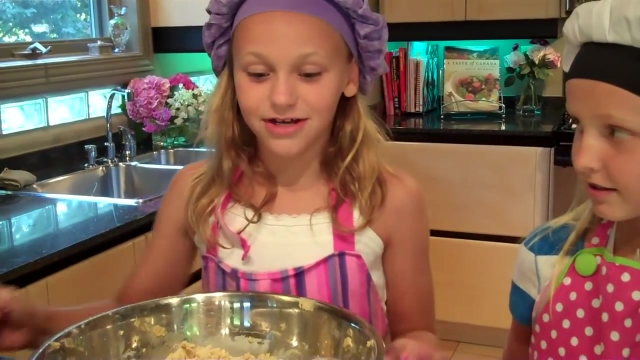 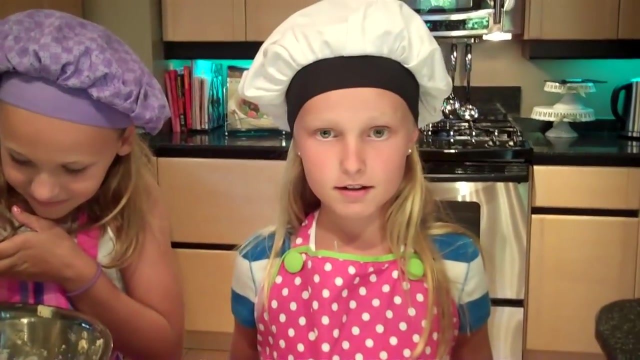 like that Oopsie doodles. So now I'm going to put it on low and just mix it in. So we've mixed all the dry ingredients and now we are going to add four generous cups of chocolate chips. A trick for cooking your chocolate chips is you put them in the oven but you don't leave. 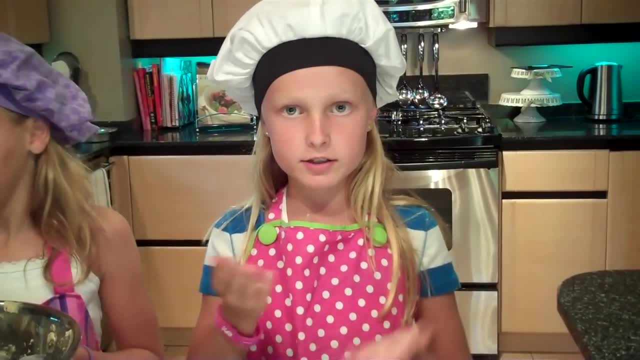 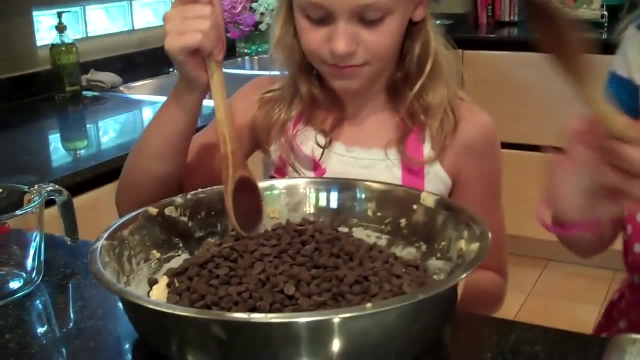 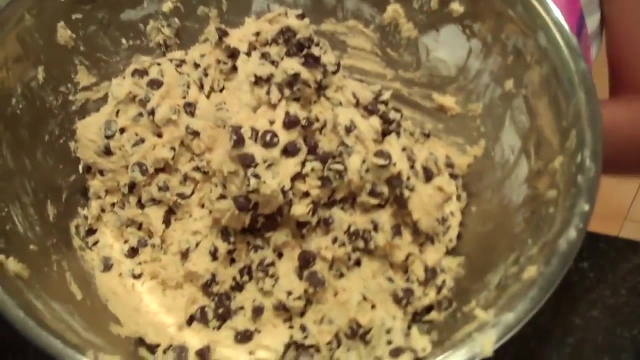 them on the same shelves. Halfway you'll switch them and you'll cook them for 20 to 25 minutes, depending on your oven. So now we are going to mix these. Okay, now we are all done mixing the chocolate chips into the batter. 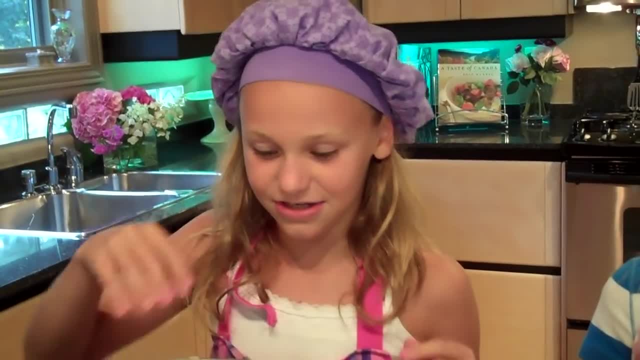 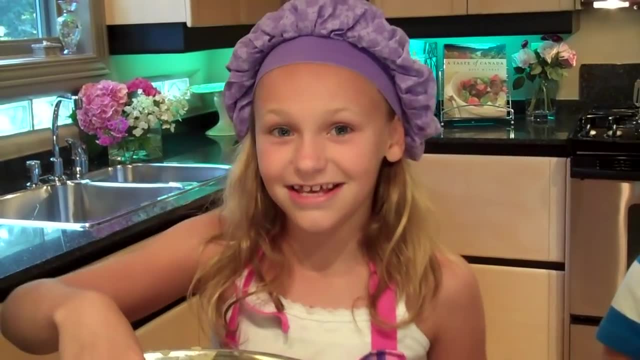 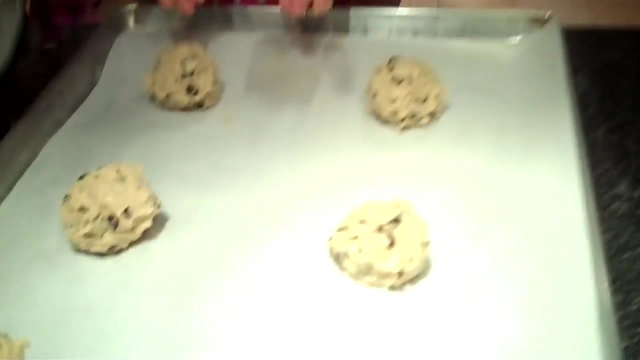 Now we are going to start rolling the dough. It usually makes about 24 large cookies. We like them big. Now see we have a little bit left. We have 24 done. Two trays are already in the oven, cooking at 350.. 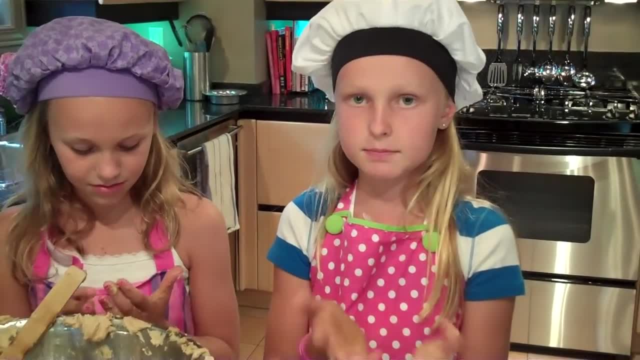 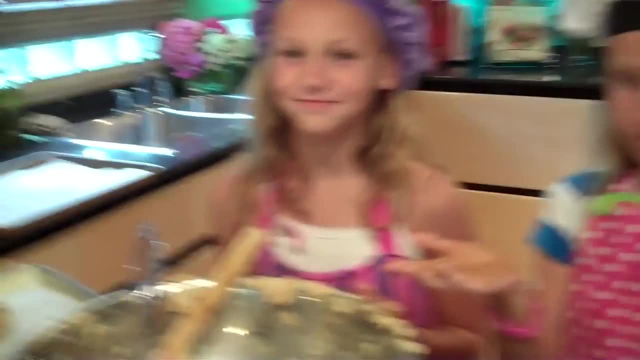 And if you like walnuts, you can add walnuts into this, but we're not big walnut fans, so we don't like them. So now, Now, my mom is letting us make two giant cookies, so we have a little bit left, so we're going. 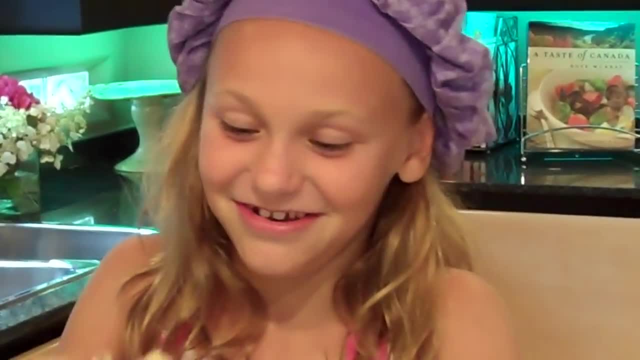 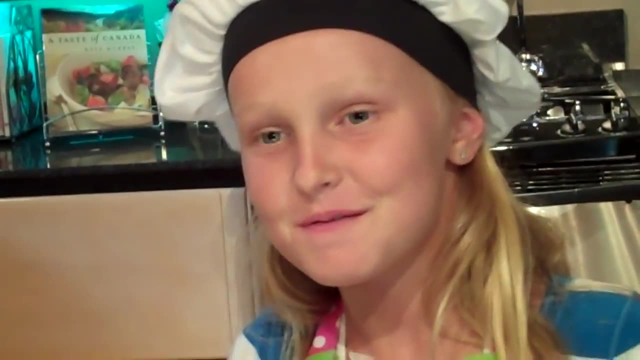 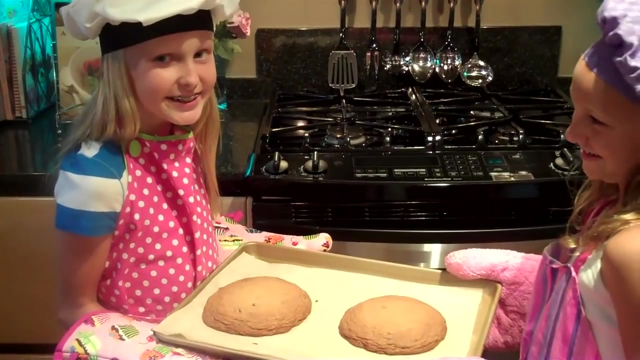 to have some fun. We're going to just make sure it tastes good. Yum A plus plus. These are our huge ones. I can't wait to eat them. They look so good because it's time to eat. I'm so hungry. 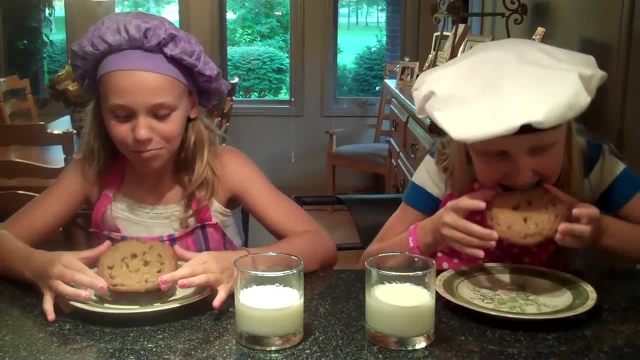 I can't wait to eat them. These are so good. These are really good- The best cookies I've ever had. Subscribe to Cooking Kids and you can get all our other videos And also leave your comments here at Cooking Kids. 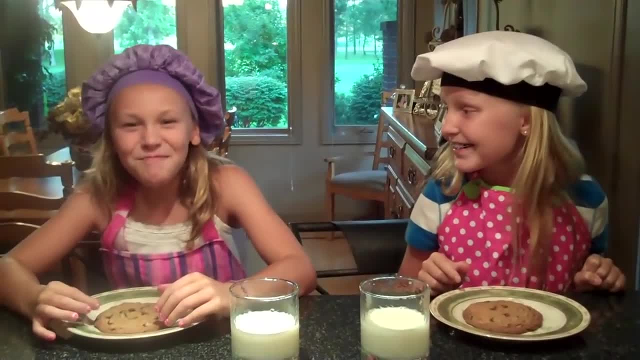 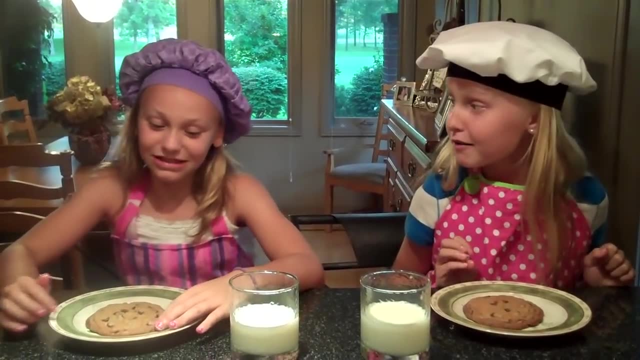 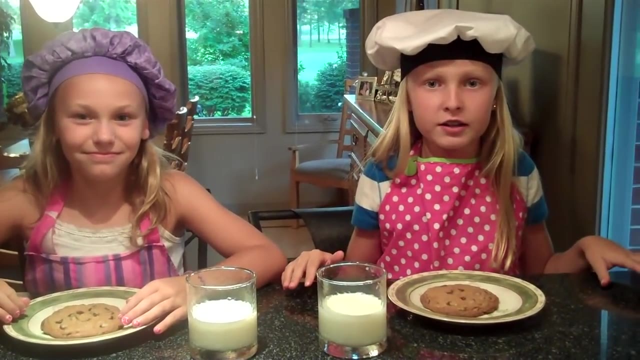 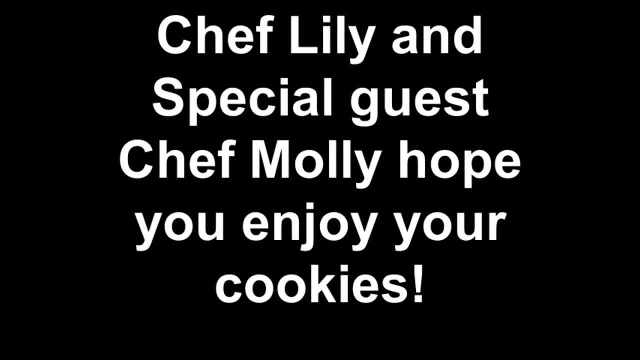